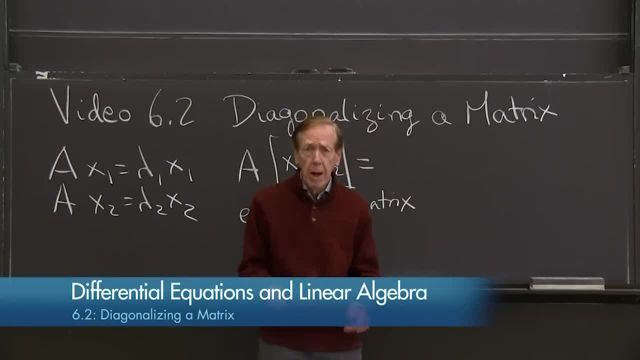 OK, More about eigenvalues and eigenvectors. Well, actually it's going to be the same thing about eigenvalues and eigenvectors, but I'm going to use matrix notation. So you remember, I have a matrix A, 2 by 2,, for example. 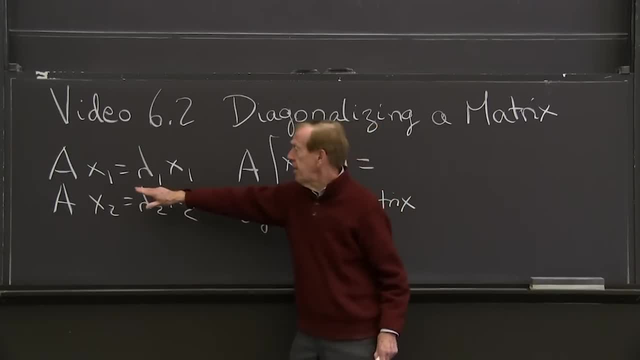 It's got two eigenvectors. Each eigenvector has its eigenvalue, So I could write the eigenvalue world that way. I want to write it in matrix form. I want to create an eigenvector matrix by taking the two eigenvectors and putting them. 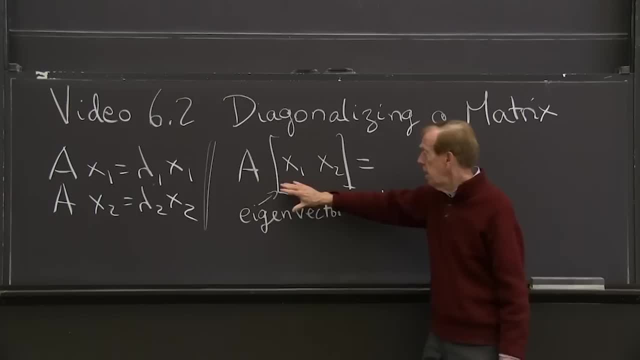 in the columns of my matrix. So if I have n of them that allows me to give one name, the eigenvector matrix, Maybe I'll call it v for vectors. So that's A times v. And now just bear with me while I. 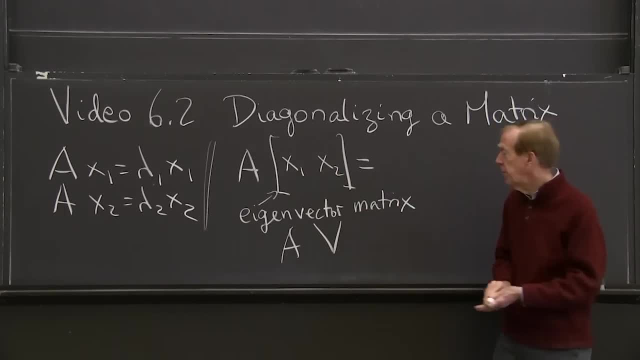 do that multiplication of A times the eigenvector matrix. So what do I get? I get a matrix That's 2 by 2.. That's 2 by 2.. I'm getting a 2 by 2 matrix. What's the first column? 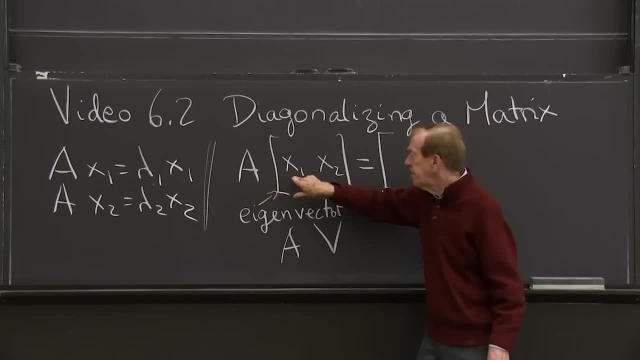 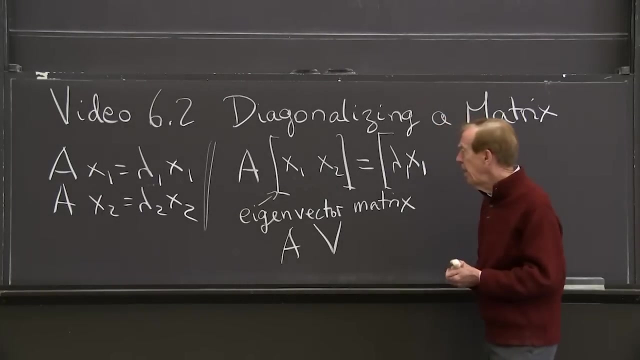 The first column of the output is A times the first column of the input. And what is A times x1?? Well, A times x1.. A times x1 is lambda 1 times x1.. So that first column is lambda 1 x1.. 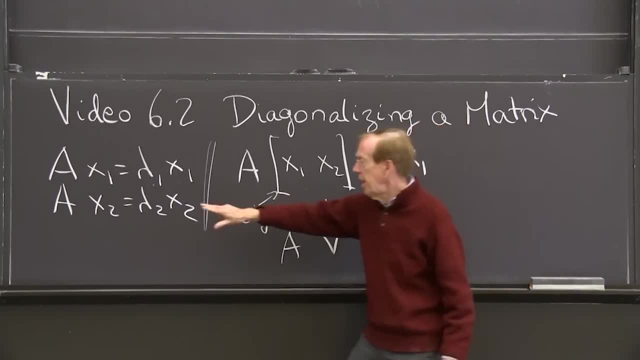 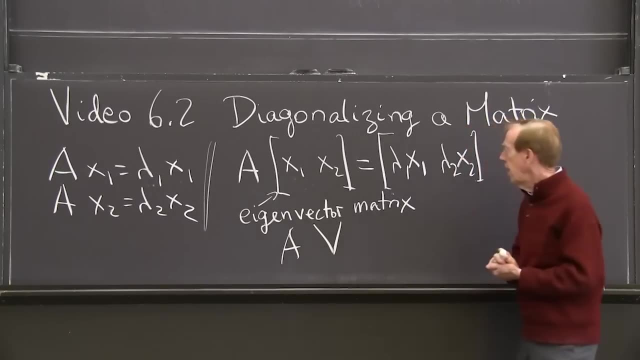 And A times. the second column is A x2, which is lambda 2 x2.. So I'm seeing lambda 2 x2 in that column. OK, Matrix notation. Those were the eigenvectors. This is the result of A times v. 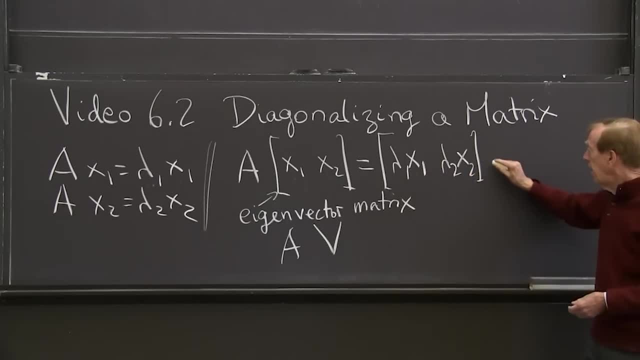 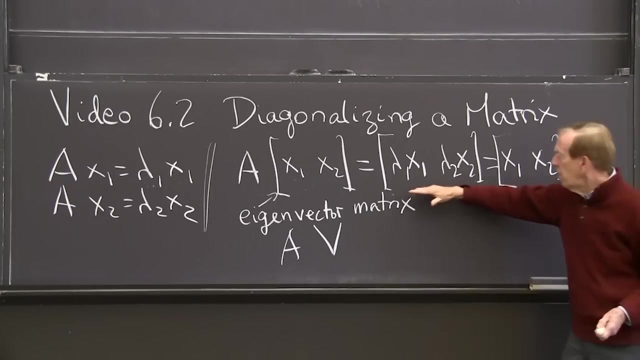 I can look at this a little differently. I can say: wait a minute, That is my eigenvector matrix x1 and x2.. Those two columns Times a matrix. Yes, I want to. I'm just taking this first column, lambda 1, x1, is 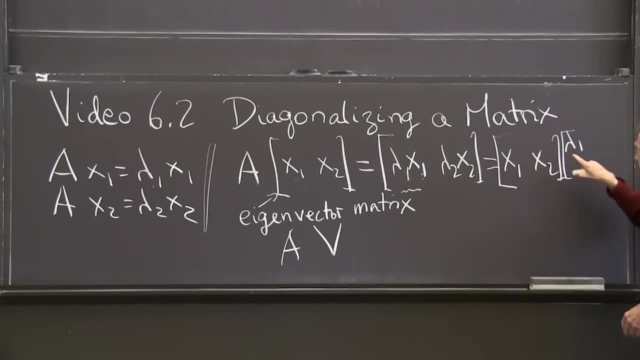 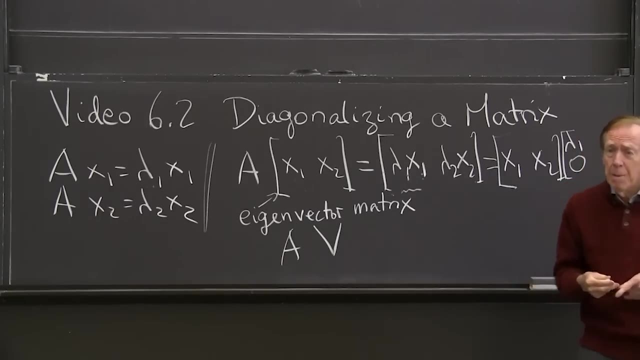 lambda: 1 times x1 plus 0 times x2.. Right there, I did a matrix multiplication. I did it without preparing you for it. I'll go back and do that preparation in a moment. But when I multiply a matrix by a vector, 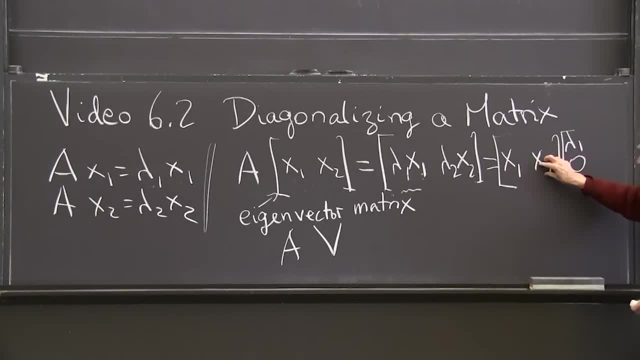 I take lambda 1 times that one, 0 times that one, I get lambda 1 x1, which is what I want. Can you see what I want In the second column here? The result I want is lambda 2 x2.. 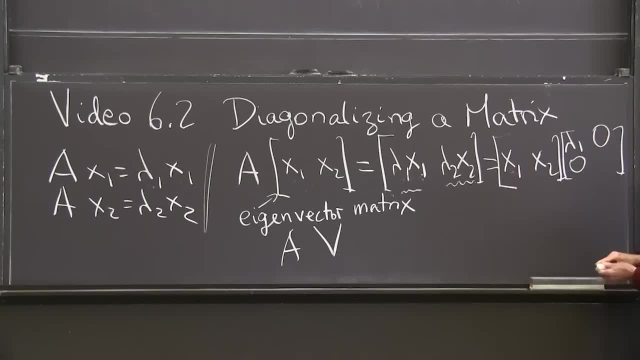 So I want no x1's and lambda 2 of that column. So that's 0 times that column plus lambda 2 times that column. Are we OK? So what do I have now? I have the whole thing in a beautiful form. 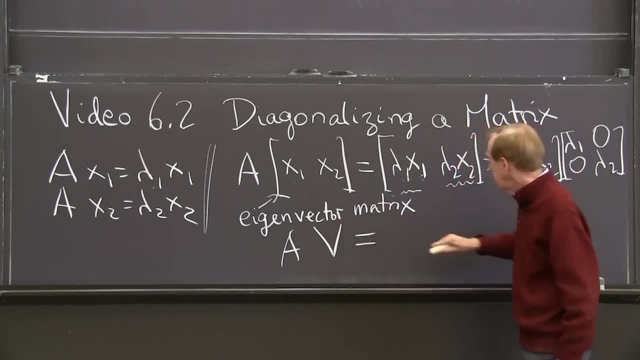 This is A times the eigenvector matrix equals. there's the eigenvector matrix again, v. And here is a new matrix that I'm going to. that's the eigenvalue matrix, And everybody calls that because those are lambda- 1. 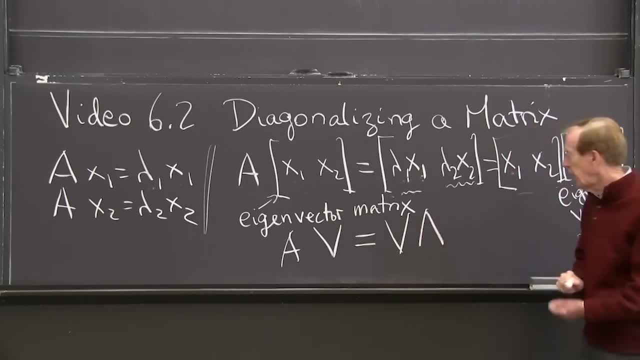 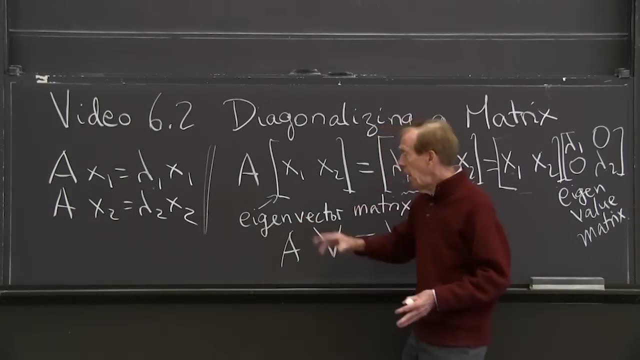 and lambda 2, so the natural letter is a capital lambda, That's a capital Greek lambda. there The best I could do. So you see that the two equations written separately, or the four equations, or the n equations combine into one matrix equation. 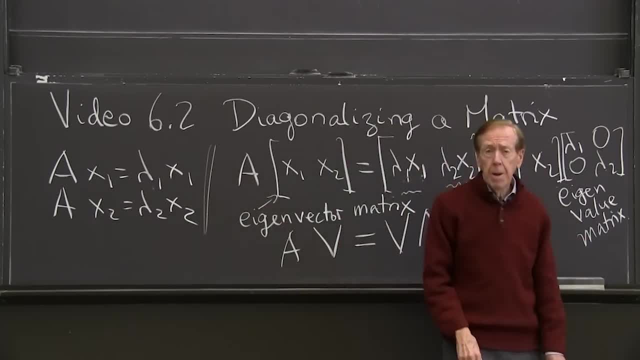 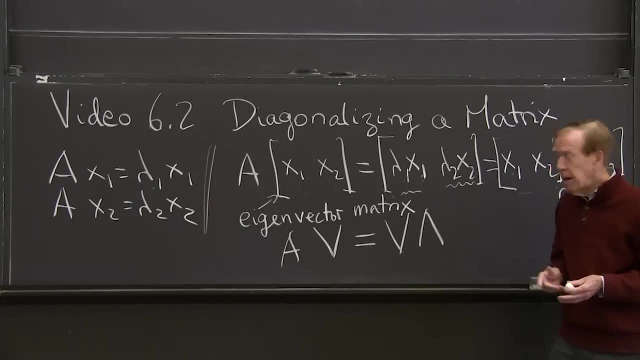 This is the same as those two together. Good, Good. But now that I have it in matrix form I can mess around with it. I can multiply both sides by v inverse. If I multiply both sides, If I multiply both sides by v inverse, I discover well. 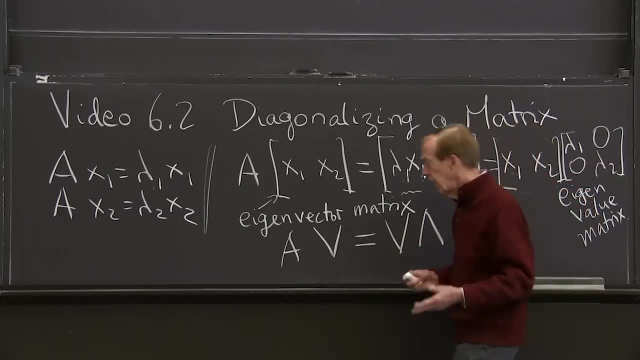 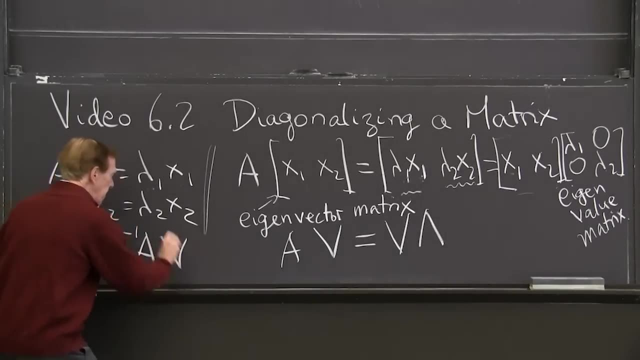 shall I multiply on the left by v inverse? Yes, I'll do that. If I multiply on the left by v inverse, that's v inverse A v. So this is matrix multiplication And my next video is going to recap matrix multiplication. 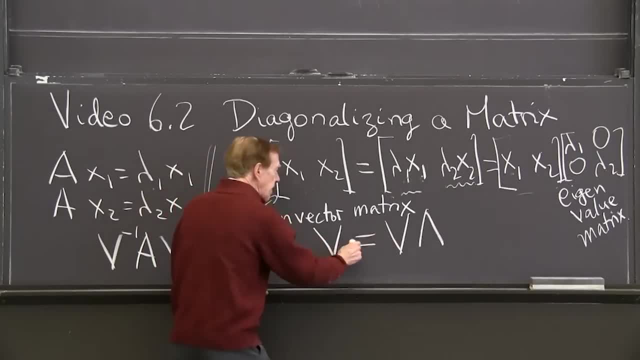 So I multiply both sides by v- inverse v, inverse v. inverse times: v is the identity. That's what the inverse matrix is: v inverse v is the identity. So there you go. Let me push that up. That's really nice. 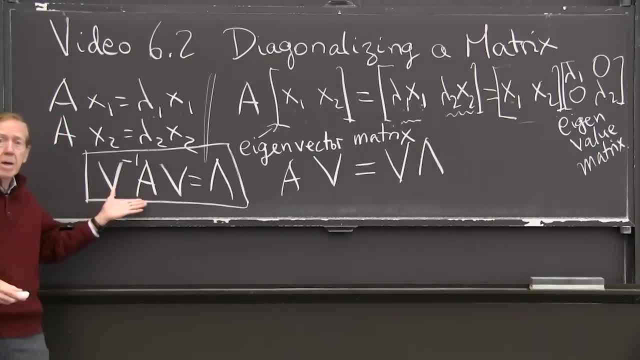 That's really nice. That's called diagonalizing A. I diagonalize A by taking the eigenvector matrix on the right, its inverse on the left, multiply those three matrices and I get this diagonal matrix. This is the diagonal matrix lambda. 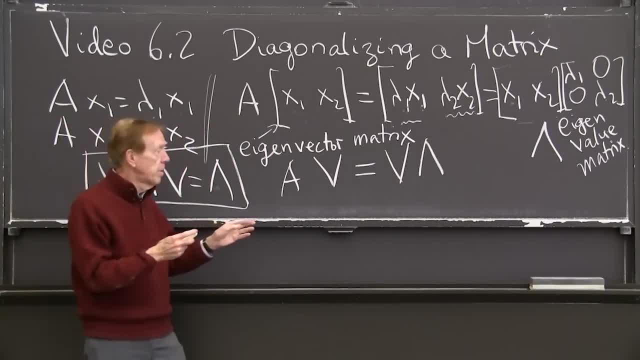 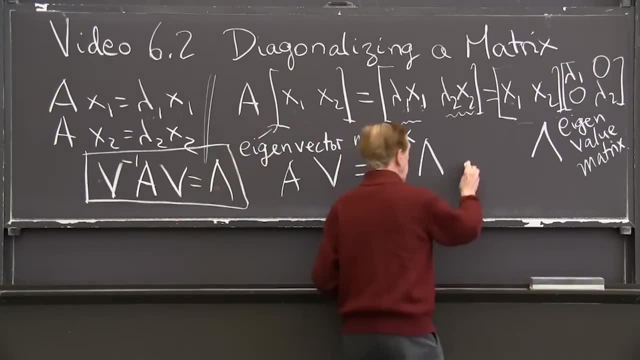 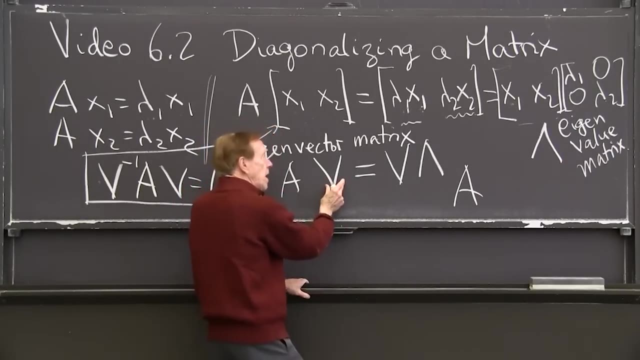 Or other times I might want to multiply both sides here by v inverse coming on the right. So that would give me A v. v inverse is the identity, So I can move v over there as v inverse. That's what it amounts to. 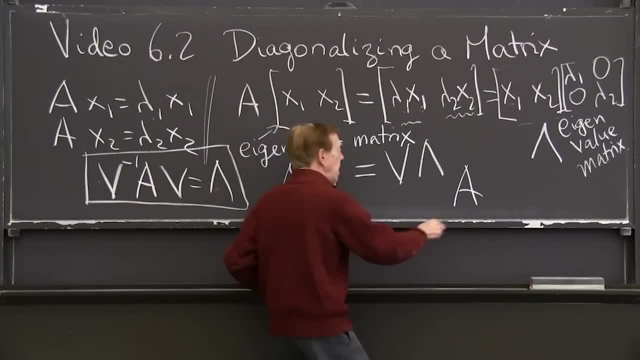 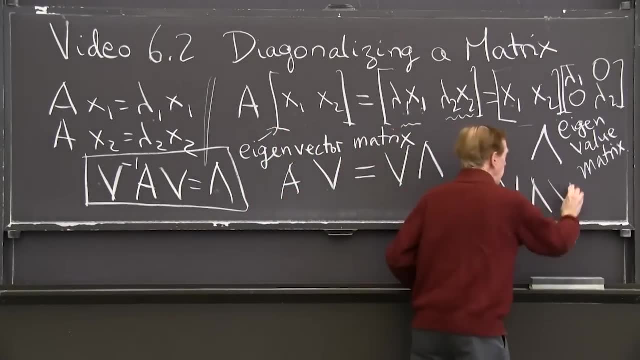 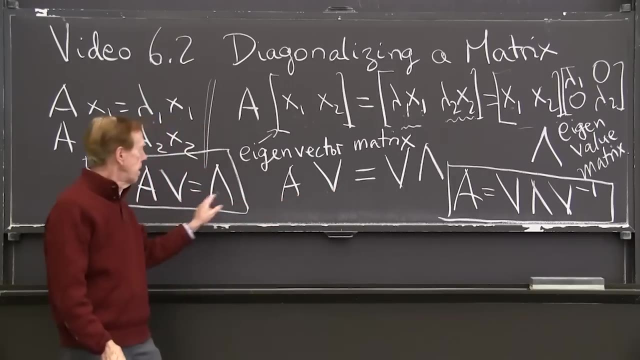 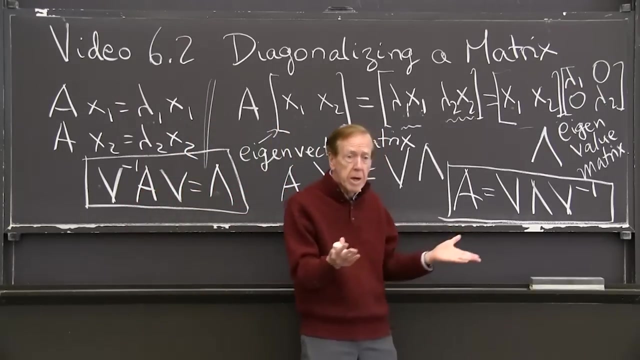 I multiply both sides by v? inverse, so this is just A And this is the v and the lambda and now the v? inverse. That's great. So that's a way to see how A is built up or broken down into the eigenvector matrix times the eigenvalue matrix. 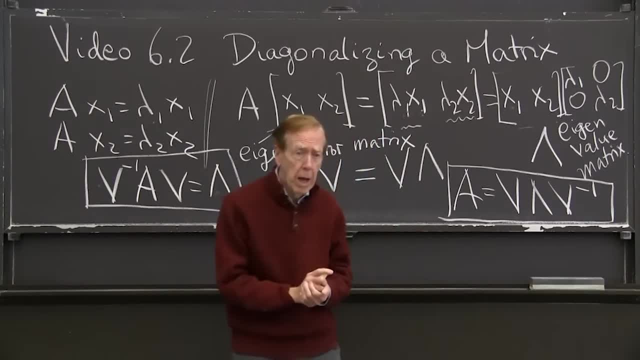 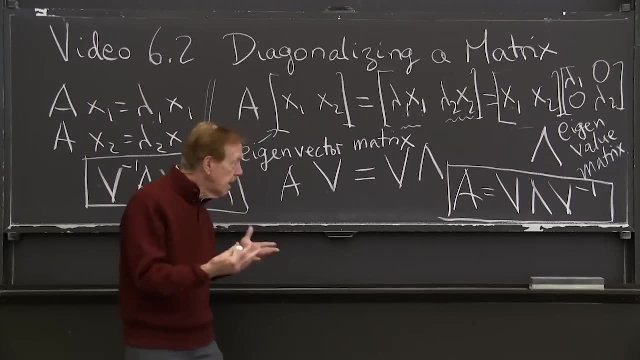 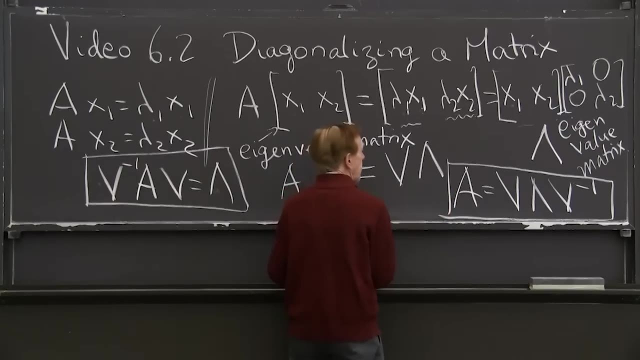 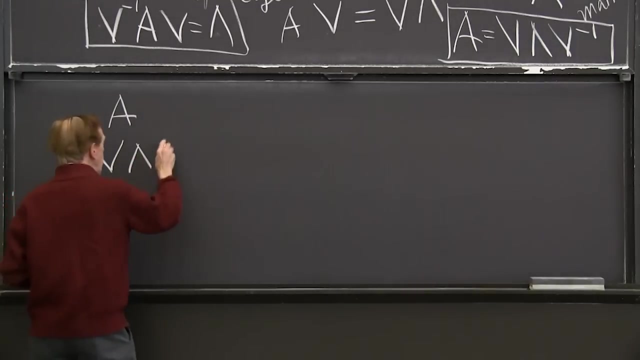 times the inverse of the eigenvector matrix. OK, Let me just use that for a moment, just so you see how it connects with what we already know about eigenvalues and eigenvectors. OK, So I'll copy that great fact that A is v lambda, v inverse. 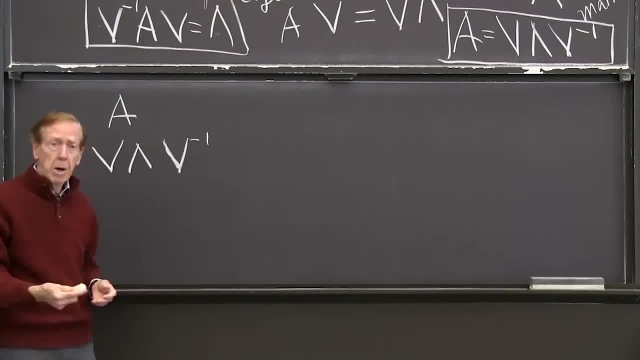 Oh, what do I want to do? I want to look at A squared. So if I look at A squared, that's v lambda, v inverse times. another one, Right, There's an A, There's an A, So that's A squared. 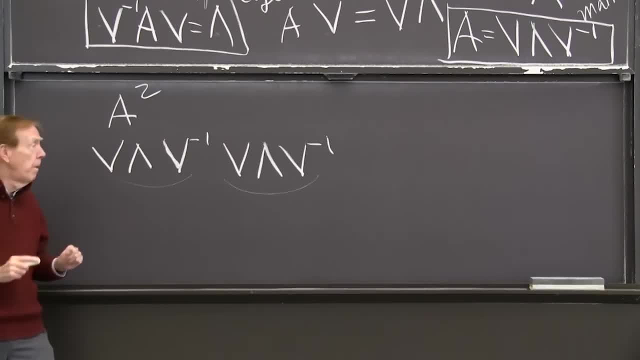 Well, you may say I've made a mess out of A squared, But not true. v inverse, v is the identity, So that's just the identity sitting in the middle. So the v at the far left, Then I have the lambda. 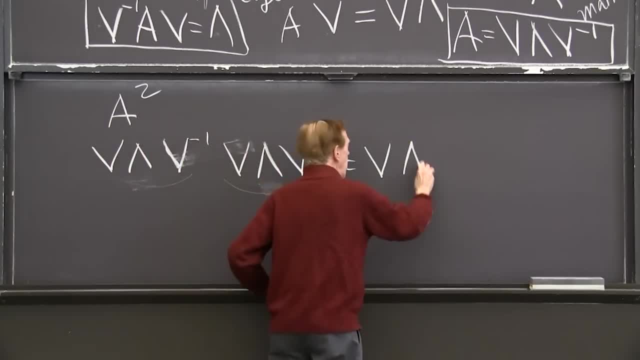 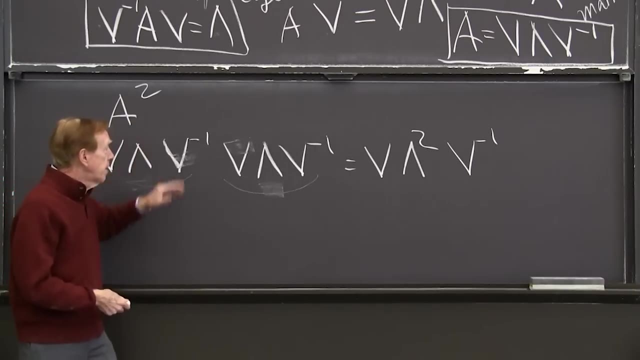 And then I have the other lambda, Lambda, squared, And then the v inverse. at the far right That's A squared And if I did it n times I would have A to the nth would be v, lambda to the nth, power v inverse. 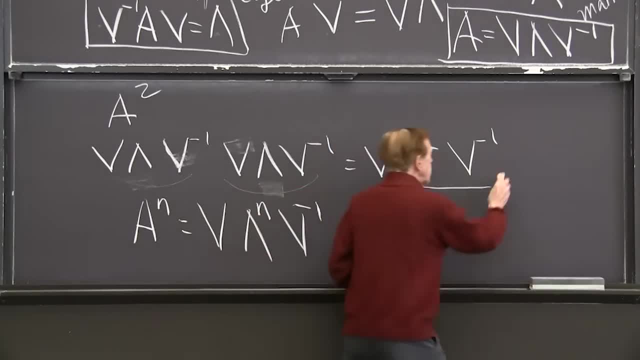 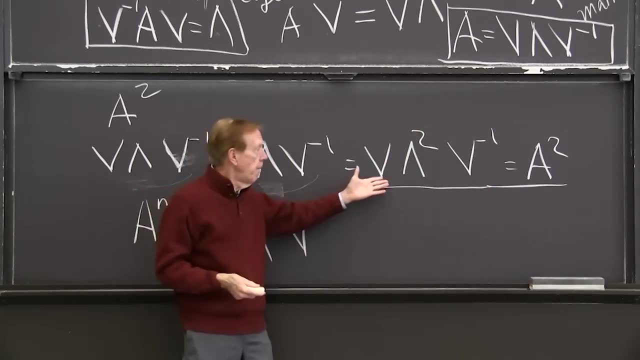 What is this saying about? This is A squared. How do I understand that equation To me that says that the eigenvalues of A squared are lambda squared. I'm just squaring each eigenvalue And the eigenvectors. What are the eigenvectors of A squared? 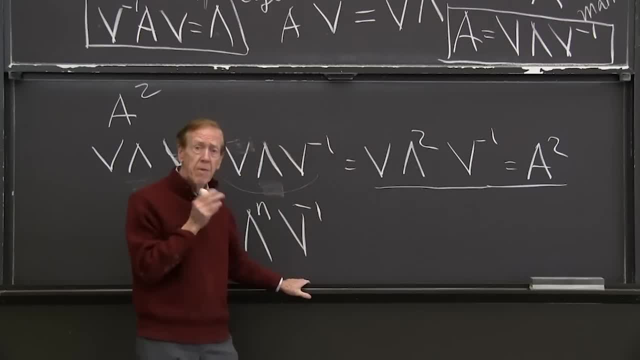 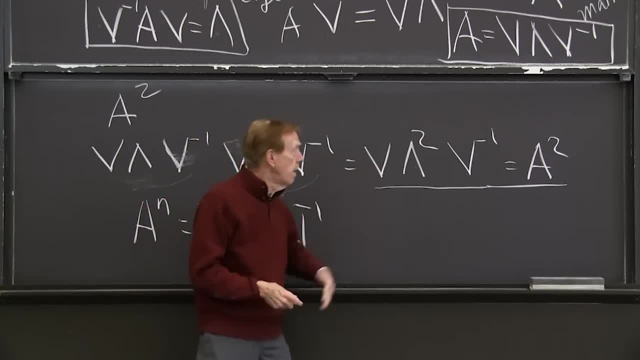 of A to the nth of A inverse, And so that's the point of diagonalizing a matrix. Diagonalizing a matrix is another way to see that. when I square the matrix, which is usually a big mess, looking at the eigenvalues and eigenvectors, 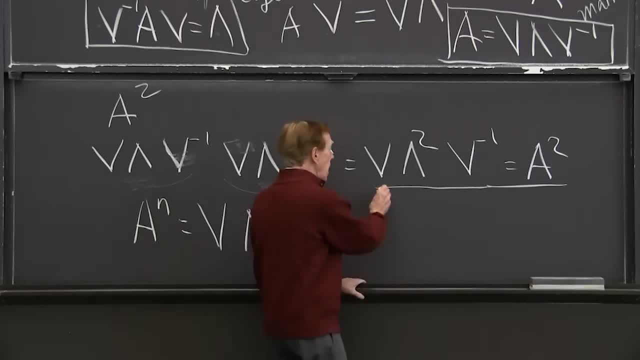 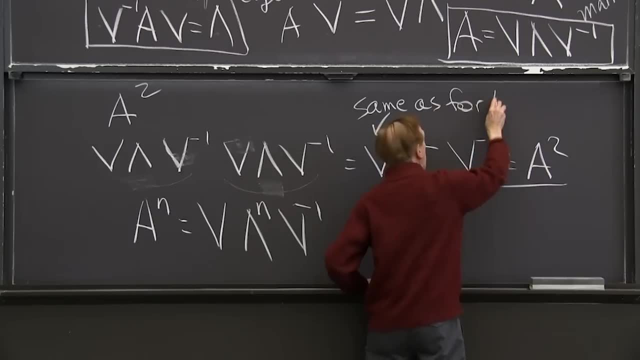 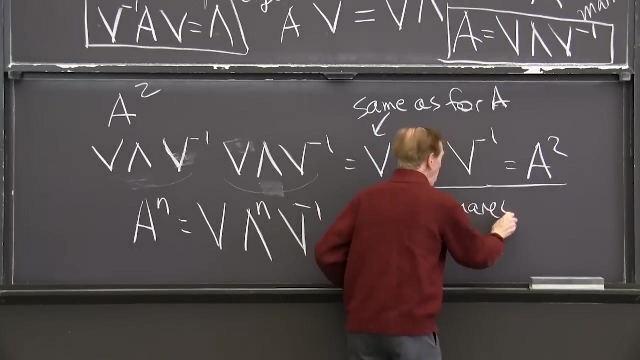 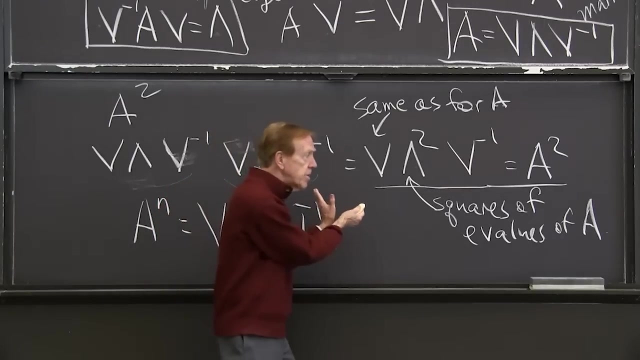 it's the opposite of a big mess. It's very clear. The eigenvectors are the same as for A And the eigenvalues are squares of the eigenvalues of A. In other words, we can take the nth power and we have a nice notation for it. 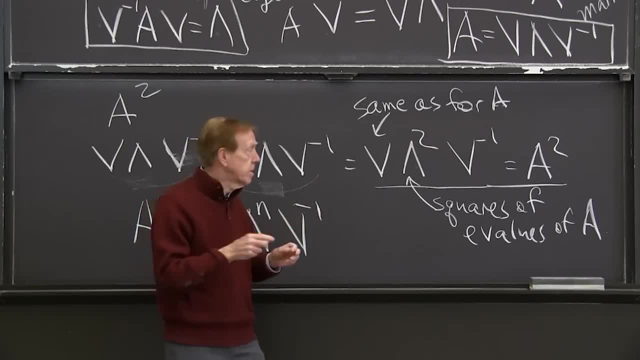 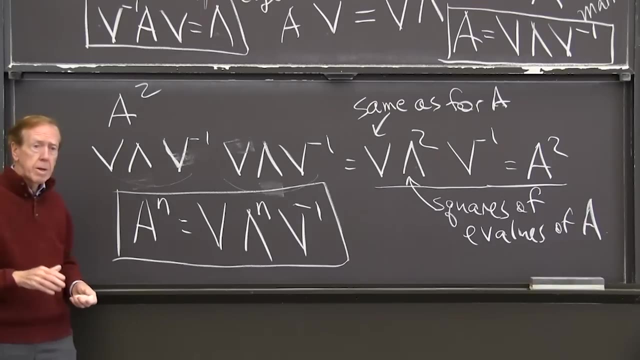 We've learned already that the nth power has the eigenvalues to the nth power And the eigenvector is the same. But now I just see it here And there it is for the nth power. So if I took the same matrix step 1,000 times.